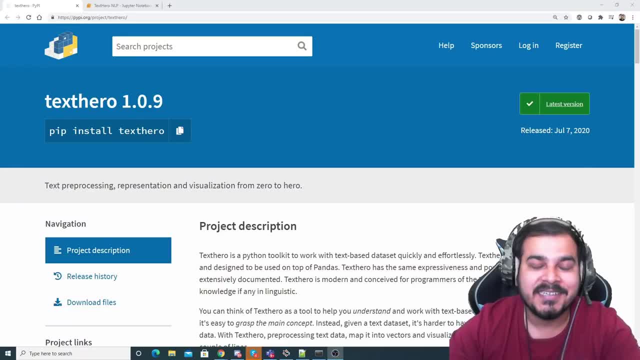 Hello all my name is Krishnayak and welcome to my YouTube channel. So, guys, today we are going to see an amazing library in Python which is called as text hero, And this is a library which will actually help you to do text pre processing, representation and visualization. So it is basically written over here in this description: text pre processing, representation and visualization from zero to hero. So we'll go through this particular library again. if you are really much interested to work with NLP, I think you've heard of various libraries like NLTK sometimes. 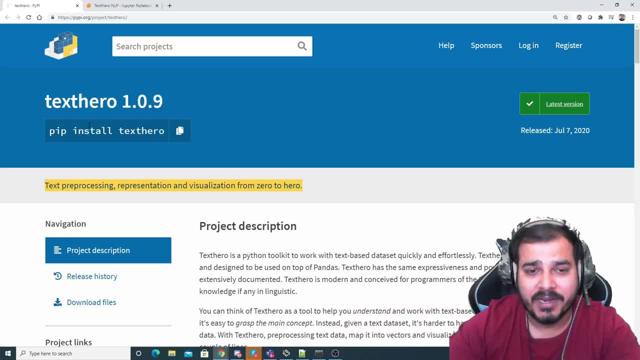 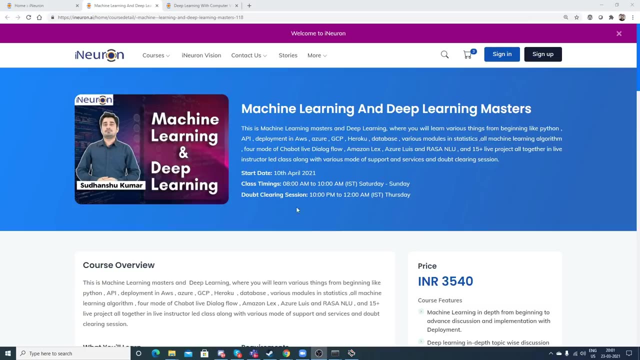 Spacey, sometimes Word2Vec, Gensim and many more things right. So by using this particular library, you will be able to do all the major tasks from all those libraries that you're probably using independently. So we'll just go through this particular library. So, guys, before going ahead with respect to this particular video, I need to announce iNeuron is coming up with the affordable machine learning and deep learning master's course, which is starting from 10th April and the timing is 8am to 10am. Apart from this, iNeuron is also coming up with the affordable 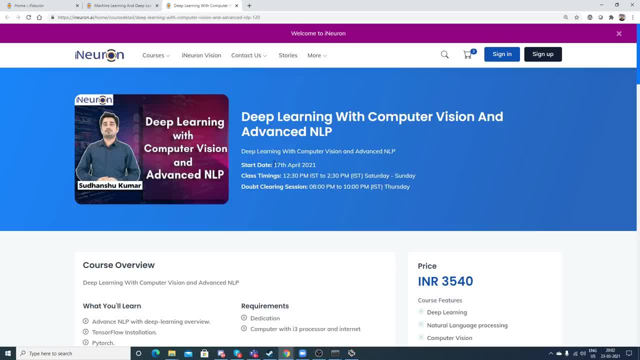 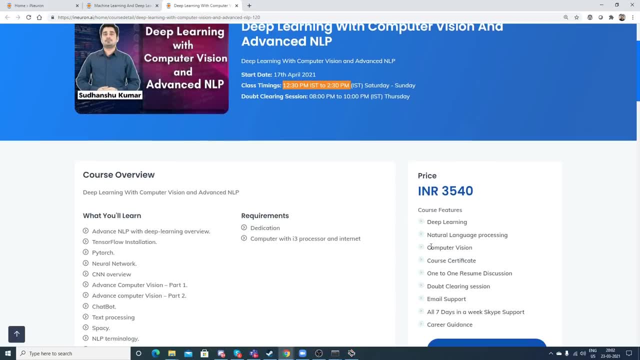 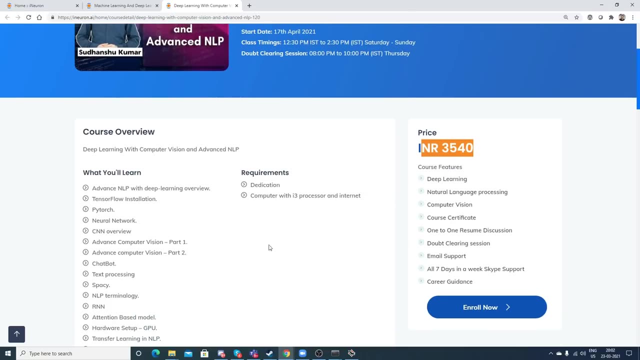 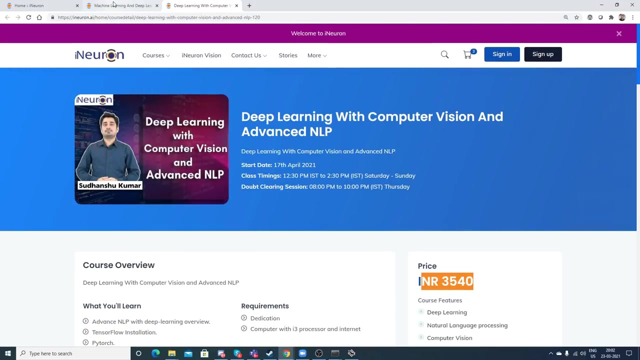 DLCV NLP course And again, this particular course is starting from 17th April 2021.. And the class timing is from 12.30pm to 2.30pm. With respect to the affordable course, guys, the course fee is 3540, where you'll be getting the entire content for lifetime. Apart from this, if you enroll also, you'll also be getting a pre recorded videos wherein you will be able to complete this particular course in fast track. Apart from this, there are a lot of features where they provide you live Skype support team. 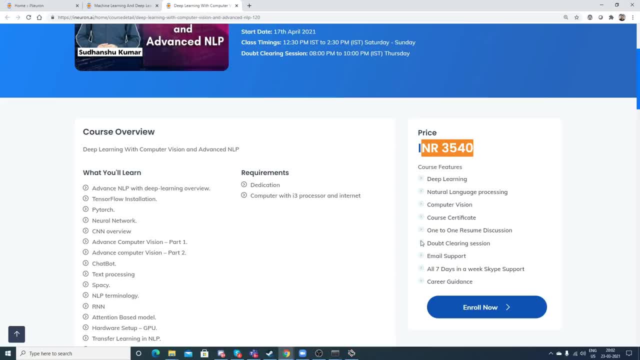 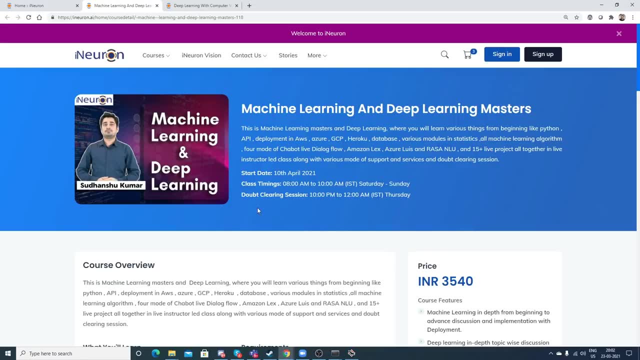 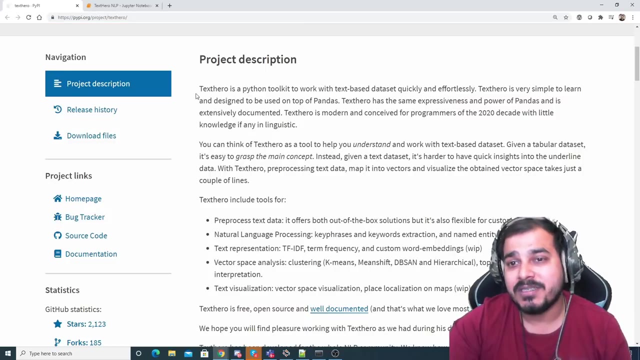 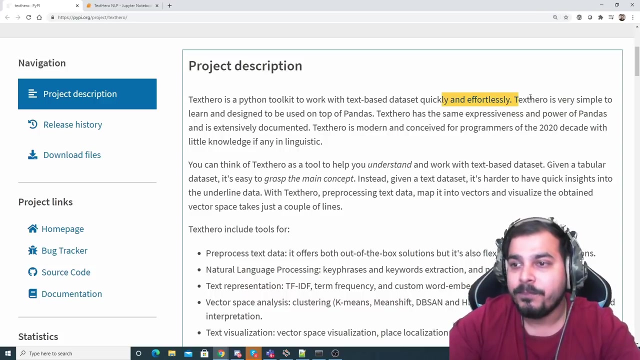 all seven days in a week, Skype support team, career guidance, email support, doubt learning session and many more things. So just check it out. all the information regarding this particular course will be given in the description of this particular video. First of all, we'll try to understand what exactly is text hero. So over here you can see that text hero is a Python toolkit to work with text data set- text based data set- quickly and effortlessly. Okay, it is very simple to learn and design on the top of design to be used on the top of Python. 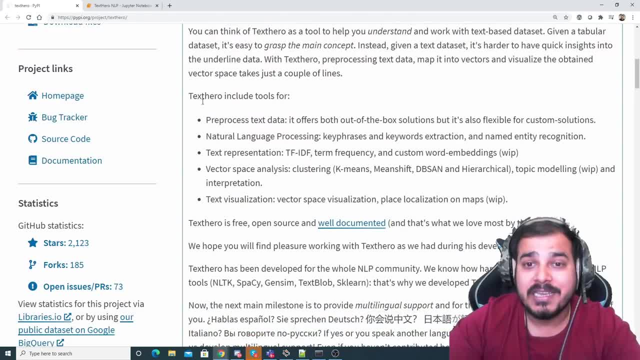 pandas. okay, so this is one of the example over here. what are things it actually includes? we'll also see a practical example for this guy, so please make sure that you watch this video till the end. uh, over here, you'll be able to see that. uh, we will be able to perform pre-processing of. 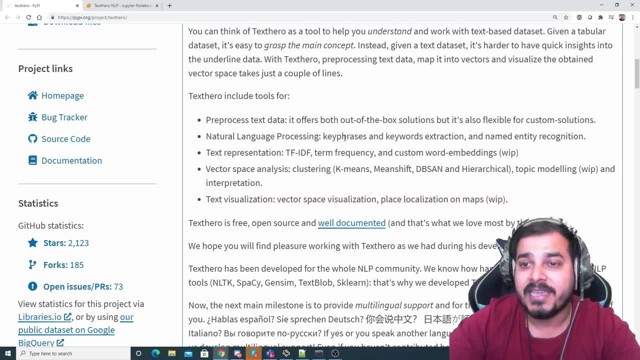 the text data, natural language processing, some of the things like key phrases, keyword extraction, name, entity recognition, text representation, like by using tf, idf, term frequency and custom word embedding. all these three techniques will be able to do it. we'll also be able to do vector space. 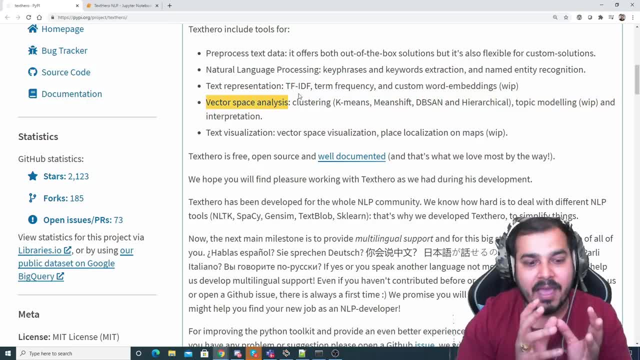 analysis. vector space analysis basically means suppose if i have a text data, i have a series of text data, i have many text data. so what i can do is that i can perform text representation over here with the help of tf, idf or term frequency or custom word embeddings, and then i can group those. 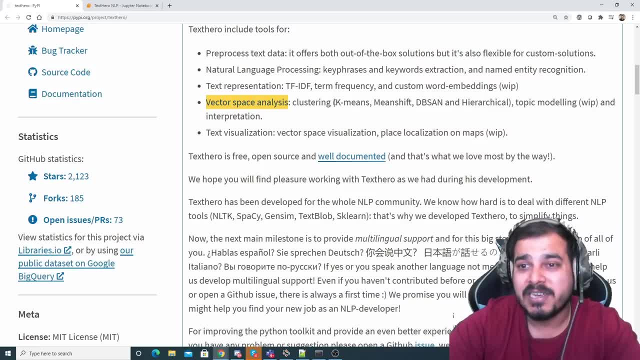 similar kind of text by using these clustering algorithms like k-means, min shift, db, scan, db, san and hierarchical right. so all these things will be able to be used to perform pre-processing, and then we also have something called as text visualization, which will actually help you to do. 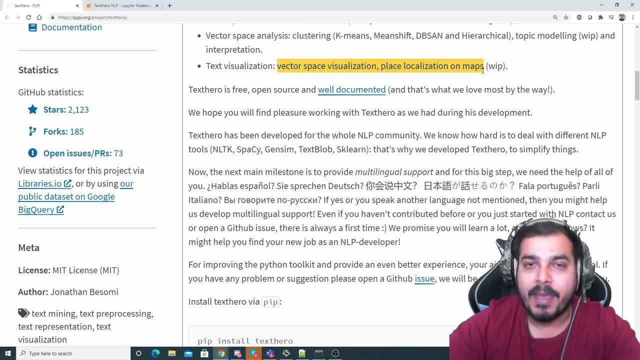 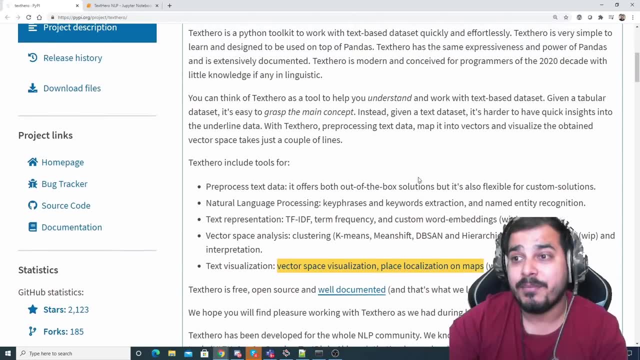 vector, space visualization and place localization on map. okay, so all these things will be able to do it. now the thing is that why is is this particular library so much important and why probably they have come up with this particular library, so here they have given this particular 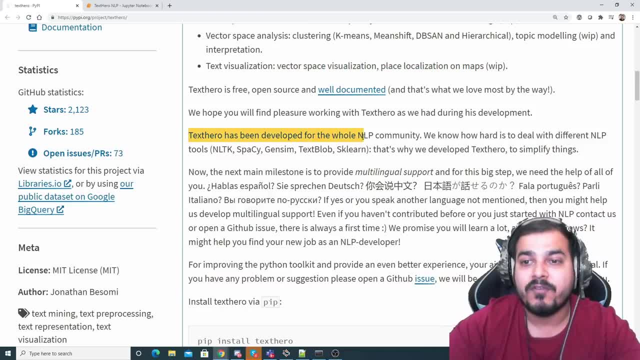 step very much easily see. this text hero has been developed for the whole nlp community. we know how hard it is to deal with different nlp tools like nltk, spacey, gen, sim, text, blob, sklearn. that's why we develop text hero to simplify things. so if you consider all these particular 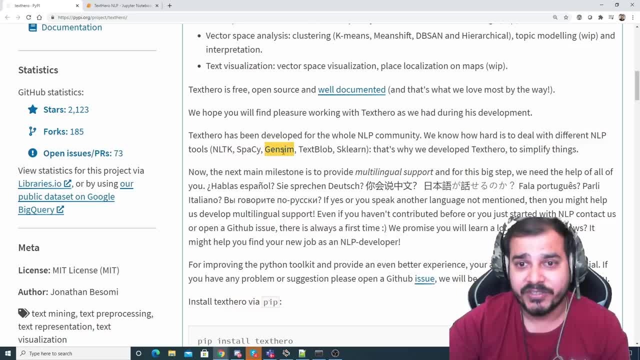 libraries, guys, there will be some unique functionalities that are probably present in gen sim. it may not be present in nltk, not be present in spacey. sometimes some other libraries may have a better performance when compared to the others. so considering this all in one for the nlp community, 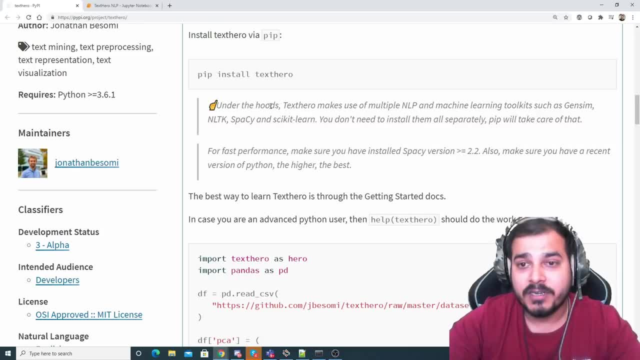 okay and uh, if you see over here guys, uh, it is also written that text hero makes use of nl, multiple nlp and machine learning toolkits such as gen, sim and nltk, skykit, learn and all okay. so, without wasting any time, let's go ahead and try to see an example. so i have given all the description. 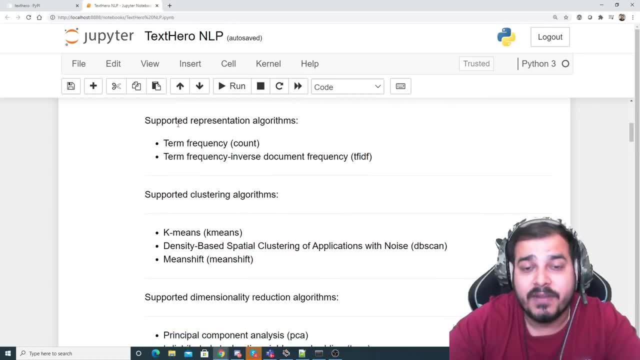 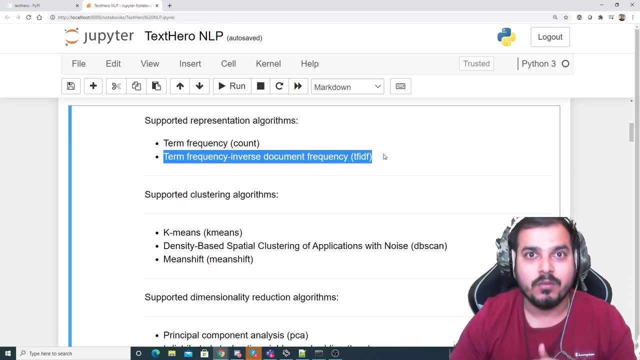 of this, what all things, what all kind of algorithm it supports? if i talk about algorithms, it knows term frequency, turn frequency, inverse document frequency, which is called as tf, idf. how does tf idf work? you can basically check out in my nlp playlist. then what are the clustered algorithms? 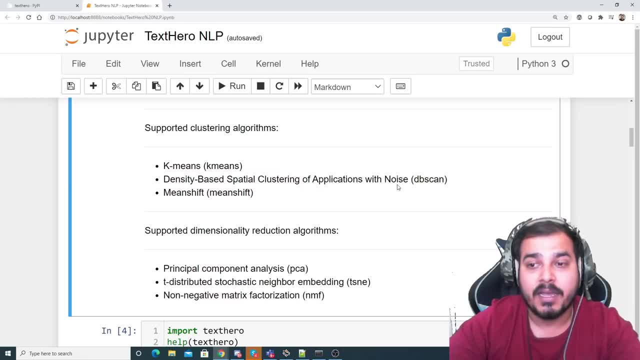 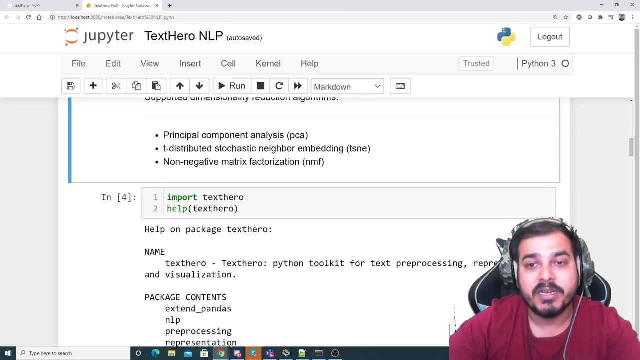 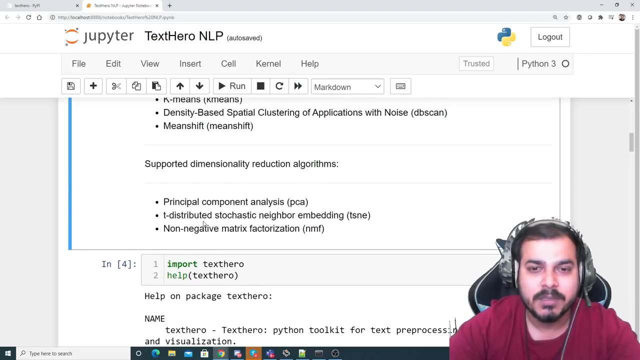 it supports k main density based spatial clustering of application with noise mean shift. then you have support dimensionality reduction algorithm. then you have pca, these distributed stochastic neighbor embeddings, non-negative matrix factorization, so all these other ones algorithms are also present in this particular algorithm. in short, it is very much important if you really, if you are using this. 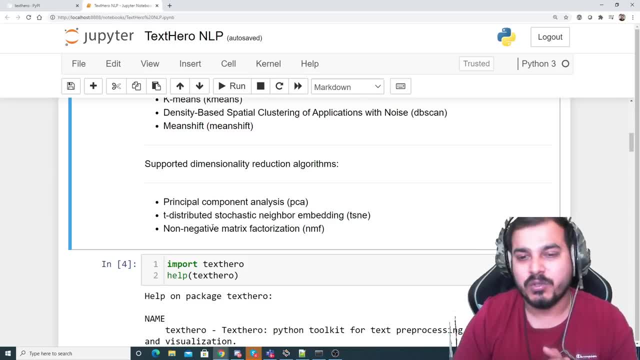 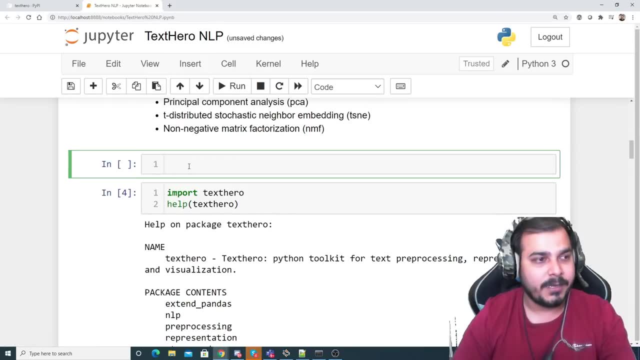 library if you are trying to do some kind of nlp task. i think using this library will actually ease in most of your tasks. so first of all, let's go and install this particular library. in order to install it, i'm just going to write something like this: okay, so i'll write pip: install text hero. okay, so once i execute it over here, you'll. 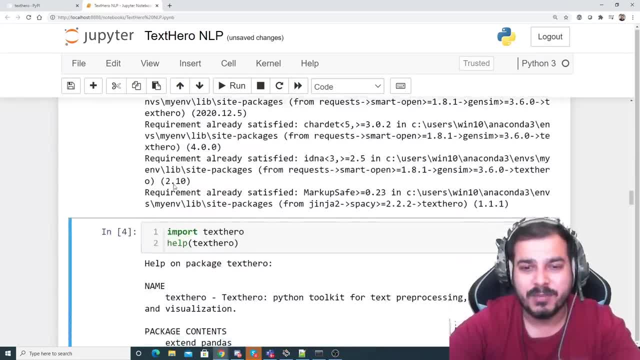 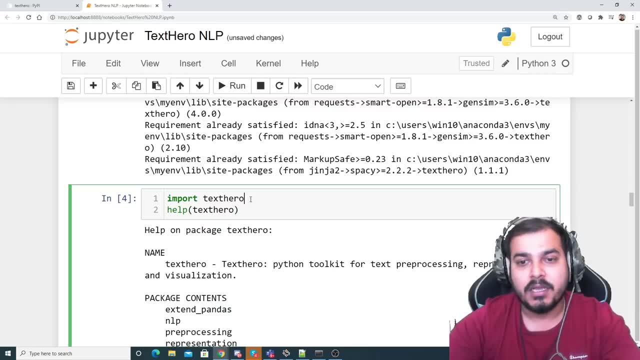 be able to see all. the requirement has been satisfied because i've already installed in this particular environment. then, if you want to see the description of entire texture, what does library, this particular library, does? you can just import text hero and just write help of text hero. so here you'll be able to see the 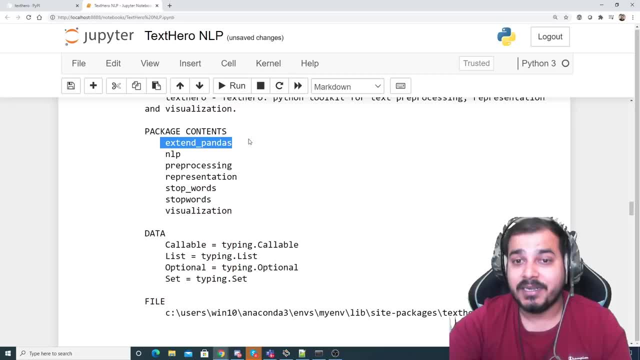 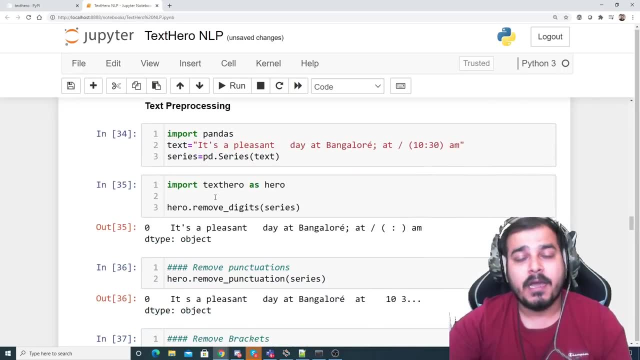 entire package, what all package content it has. uh, like it has an extended feature of pandas, nlp, pre-processing representation, stop words, uh, visualization, many more things. okay, now let's see some of the example of text pre-processing. what i can, what we can actually do: uh, one thing. 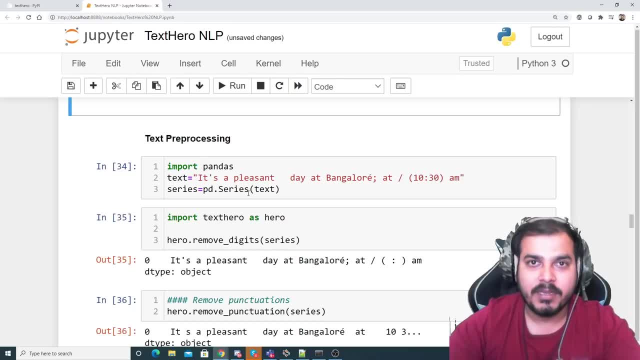 that you have to note is that, guys, whenever you want to apply a text hero, probably you will be applying on a series of text data. okay, uh, you cannot just take a string and apply it. instead, you convert. you take that whole text, convert into a series and then you 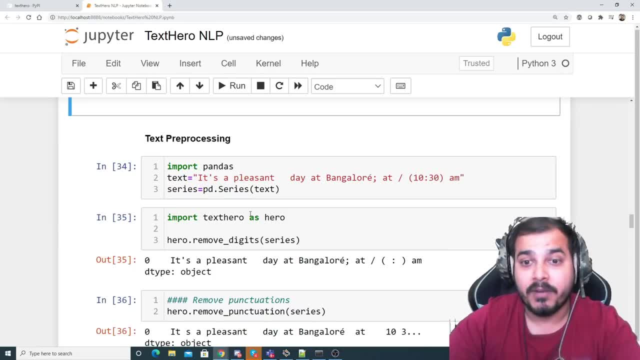 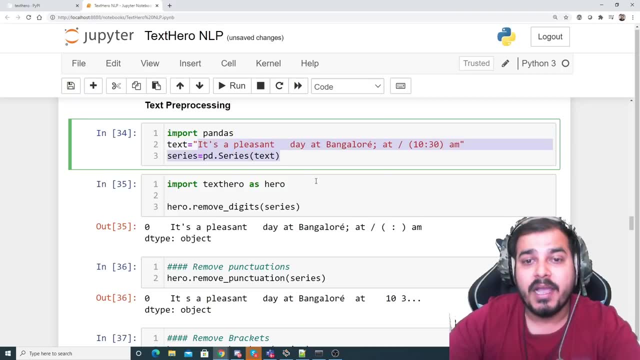 probably apply this kind of all the functionalities that are available in the text. so over here you have import pandas. here is your text. it is a pleasant day at bangalore and then we are just writing pd dot series where i'm converting the text into series. so here is. 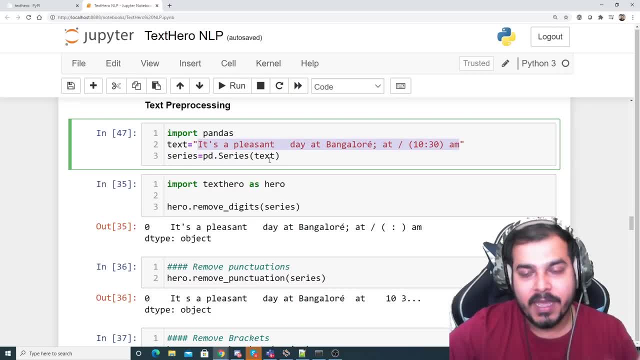 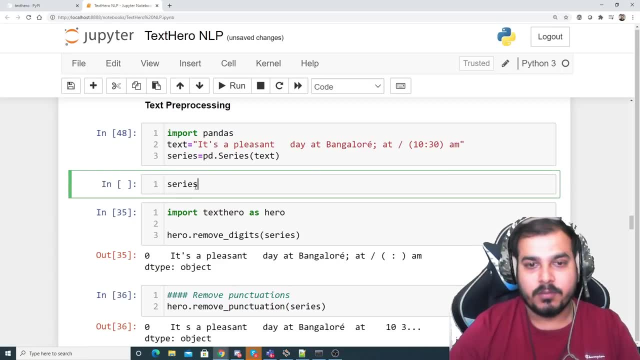 our text and we are just applying pd dot series, where we are converting this text into series. so once i execute it. so after this, i'm just going to go to my next line and probably show you this. so here is my series, which is with my index number zero. 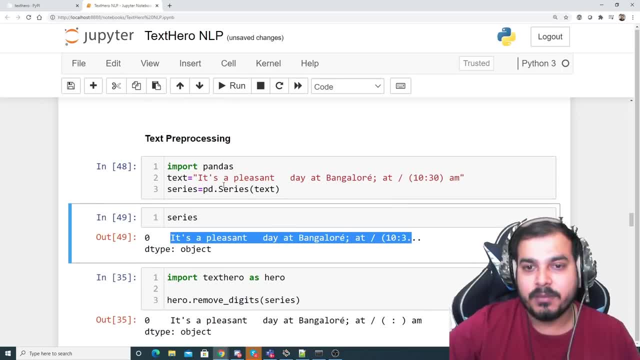 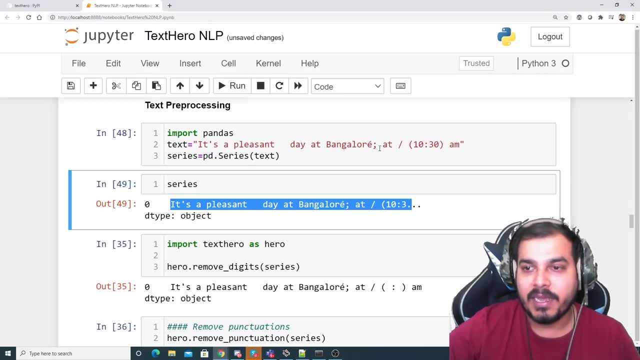 for the row, and this is my entire text. the text is pretty much simple. it's a pleasant day at bangalore at 10: 30 am. here i have also used some of the special characters over here, like semicolon, inverted commas, slash forward, slash, many thing as such. okay, just to show you that. how does it? 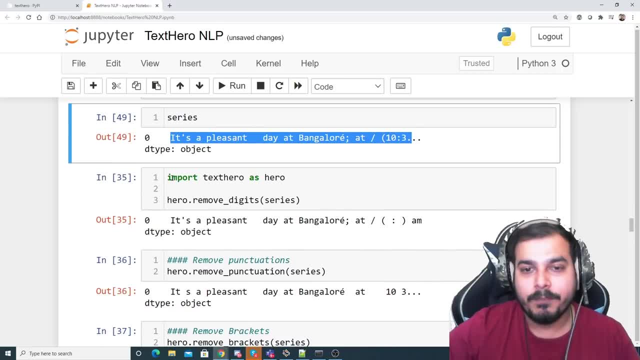 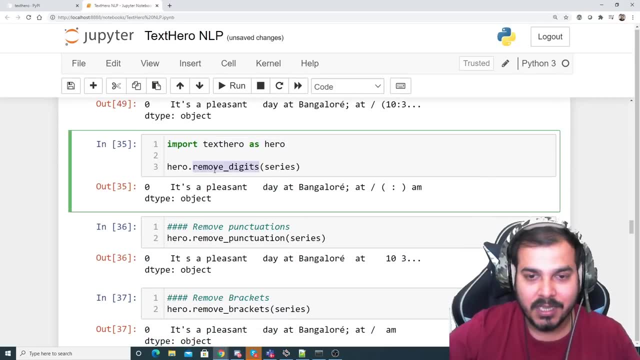 perform with respect to this kind of data. now, i'm just going to import text hero as hero. after this, the first inbuilt function that i'm going to discuss about is something called as remove digits. remove digits by default it will. you don't have to write a for loop on the entire series, just 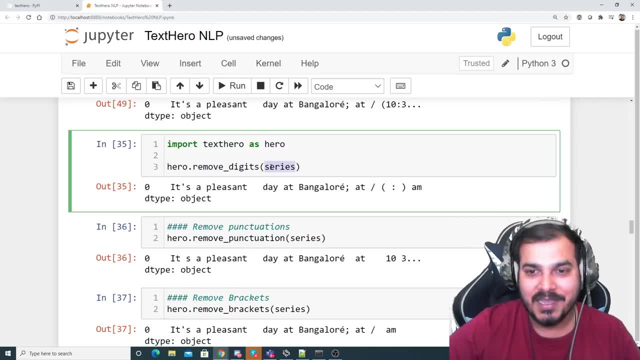 it will be acting on the entire series, on all the rows of the series, because when i was previously showing you some of the videos in nfp, we used to iterate through each and every row and probably do all the pre-processing. now, just by using this inbuilt function and giving the series automatically, 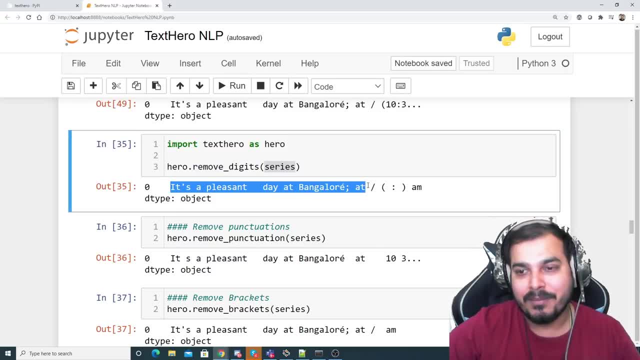 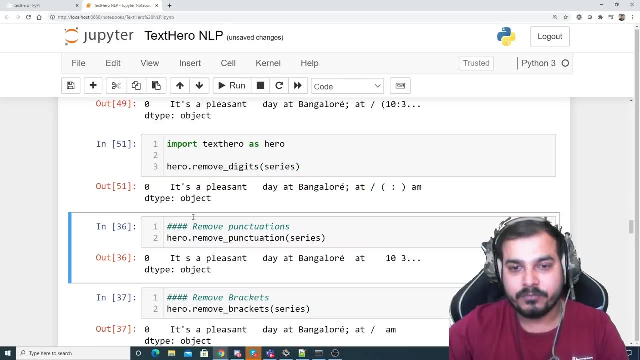 it will be able to perform it. so here it shows: it is a pleasant day at bangalore and it is just removing all the digits. okay, so once i execute this, this works fine. so here you can see. there will be some warnings coming- uh it, you not worry about it either- that particular versions may get. 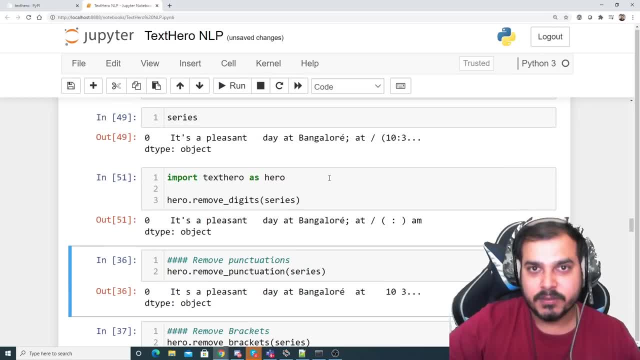 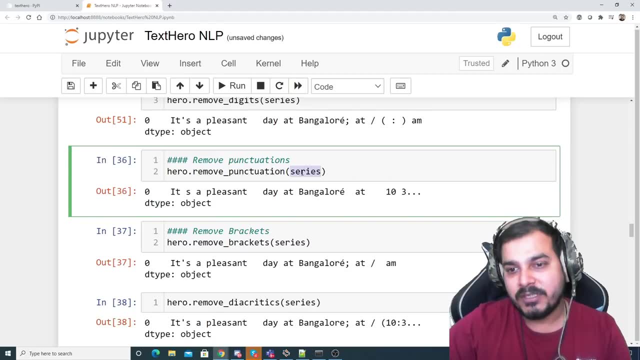 deprecated and a new functionality may come. if there is any such situation, i'll let you know. okay, then there is also an inbuilt function which is called as remove punctuation. so if i'm using remove punctuation on series, i'll also be able to execute this. so here you can see that all the punctuation will be gone. 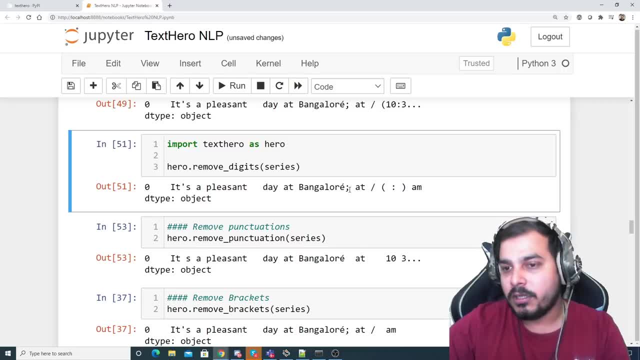 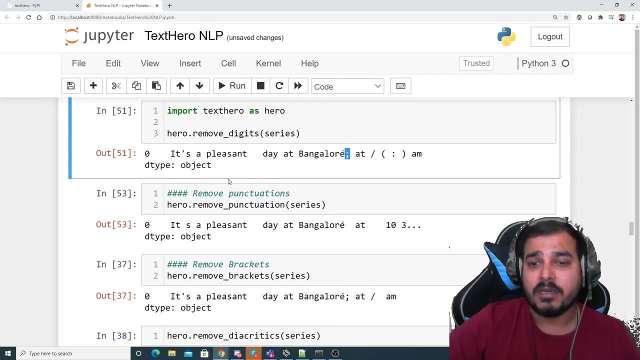 this will be gone. semicolon will be gone in all the uh, this, uh, all all the special things has just got removed. see over here: uh, this quotation has also got removed. guys, if you see this entire thing right, this quotation, semicolon, inverted commas, everything has got removed. okay, so that is what it says: remove. 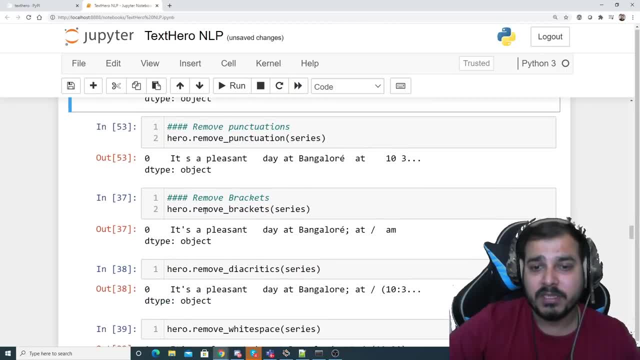 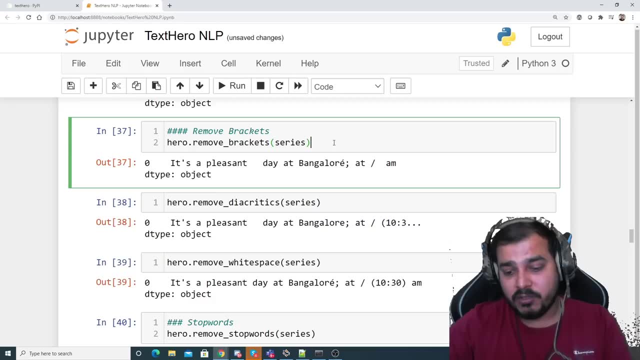 punctuation. now, after this, you will be able to see that we also have an inbuilt function which is called as remove brackets. if there is any brackets in the sentences, we can remove it. so, in this way, what we will have here is an inbuilt function called as remove punctuation. so in this way, 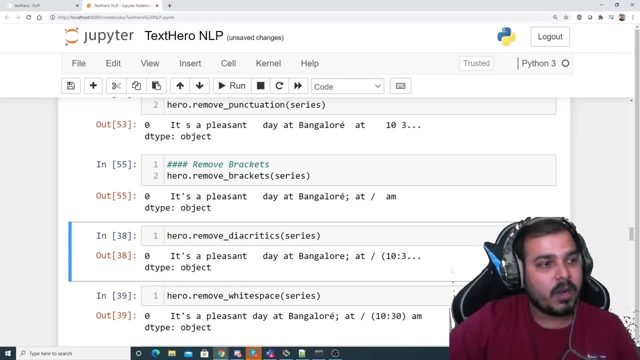 we can see that a moment. the minute you remove the pactu or the inboxуть is removed, you will probably go back to. if we want to remove it now. as i'll, alrighto, back to the first one, which was that of how i'm checking and gauge and how to are going to be able to remove coherent. 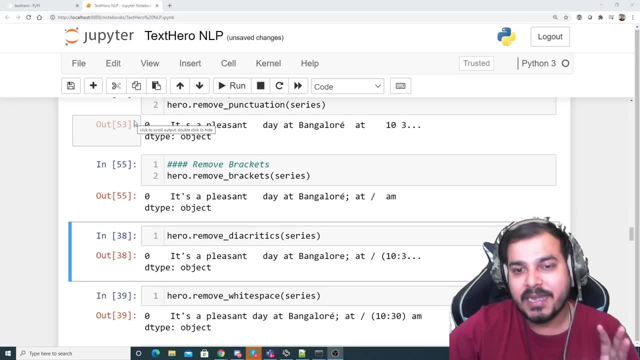 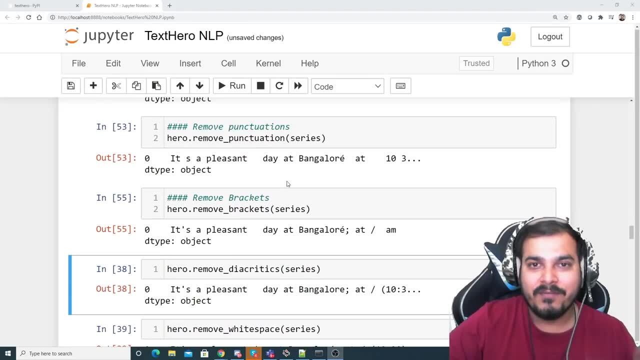 things. okay, as per the above, i will probably do it with just the same use, but again, that will take a little while, like it will take some some time, but it has no problem right now, but promised i will. i'll also show you one function which will do all these things also, guys. 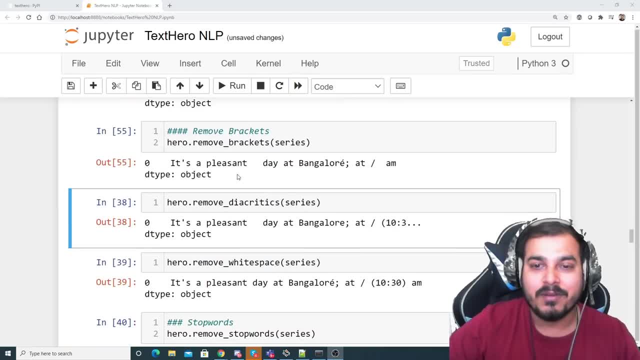 punctuation, brackets, everything, digits, everything. it will be do. there is also a function which is called as remove die critics in this particular function. here you will be seeing that suppose i can see bangalore, the word over here on top of e. there is a special character something. 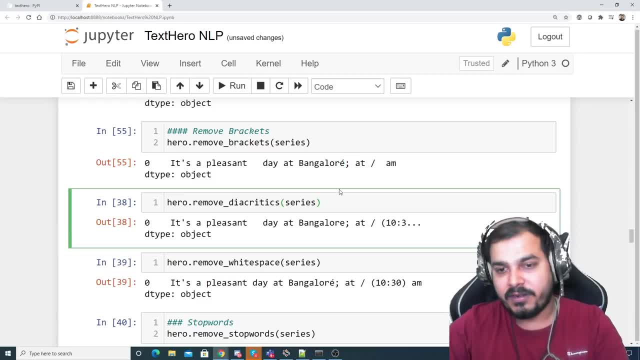 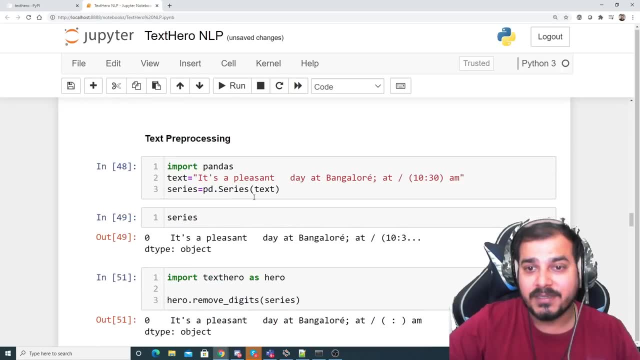 like this, it will be able to remove this kind of words also. so if i try to execute it here, you can see now i'm getting something like bangalore. okay, so all these things are there. you can also remove white spaces here. you can see that i've defined a white. 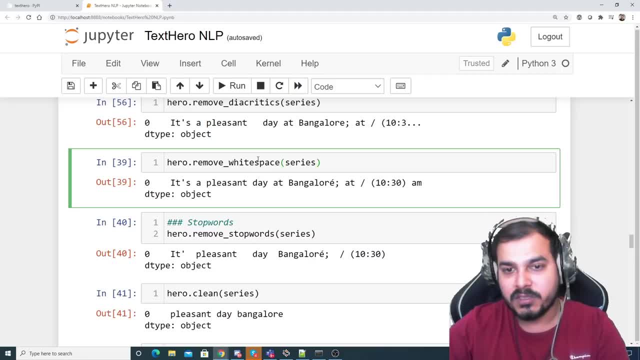 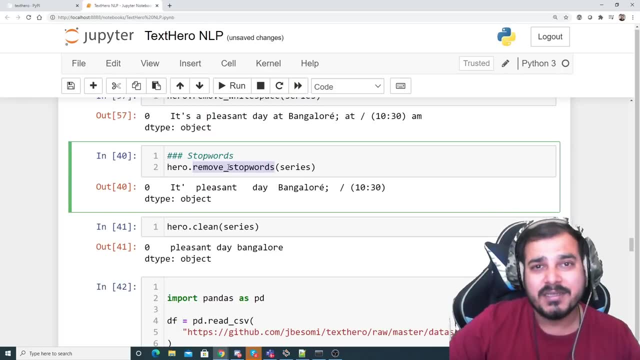 space over here. if i want to remove white spaces, i can use this inbuilt function called as remove underscore white space. similarly, if i want to remove stop words- stop words basically means all the simple words like the off, he, she, not this, that, that, this right, all the. 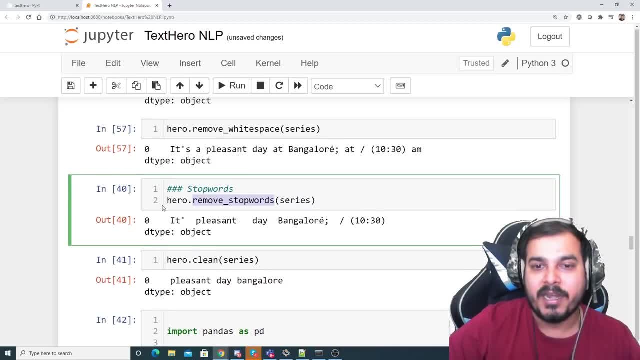 stop words can also be removed with the help of this particular library. so i'm writing hero dot remove stop stop words on series and automatically everything will get removed. so you can see: am is not there. uh, it has become it, you know, because it was after this particular uh single. 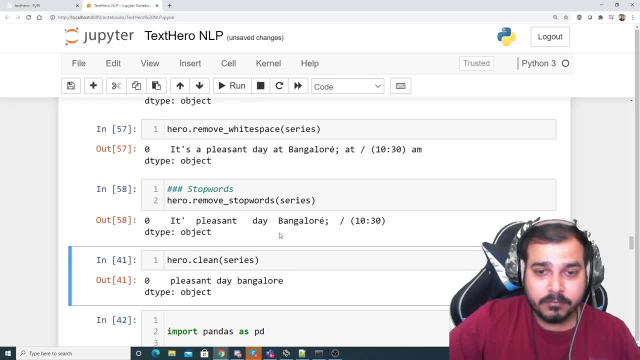 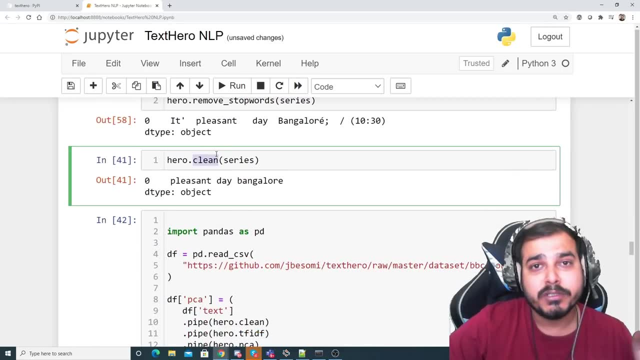 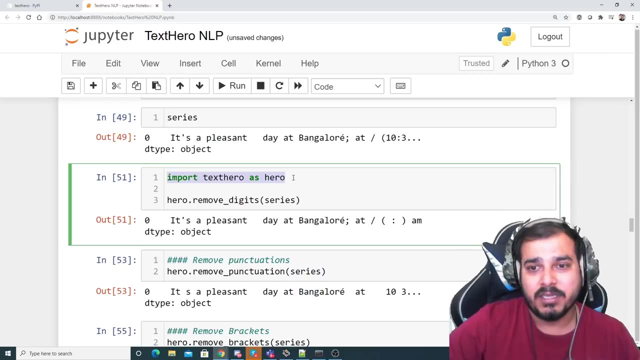 inverted comma. the s was there. it has got removed. now suppose i want to uh apply all these functionalities. uh, inside this i can also use a function which is called as clean heroclean. remember, hero is nothing, but i'm just importing from here: import text: hero as hero right. 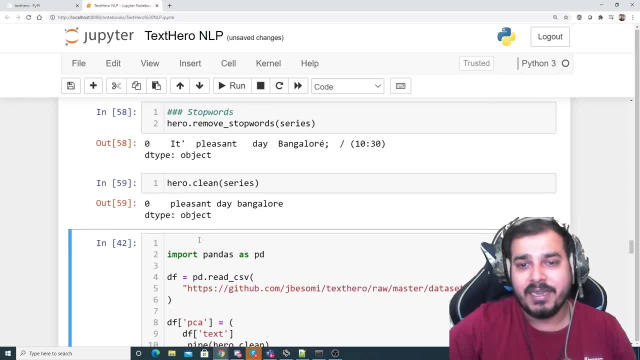 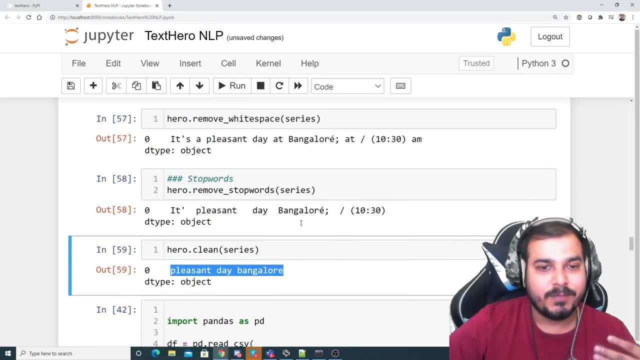 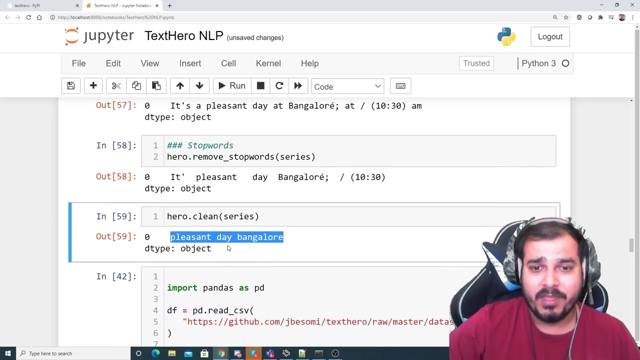 so here you can see heroclean on series. automatically you'll be getting a very simple statement: pleasant day, bangalore. probably over here. you can see that some kind of pre-processing has happened inside it, where it is just removing all the special characters, and it has clearly cleaned this particular data. 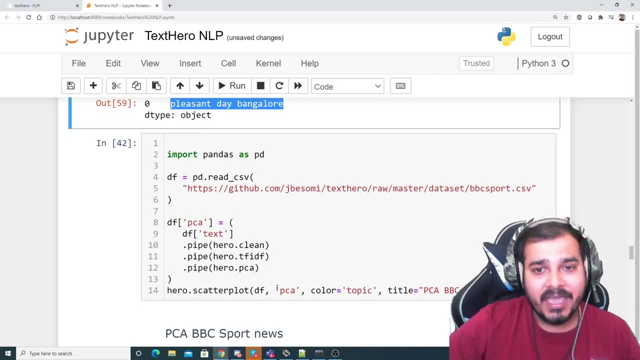 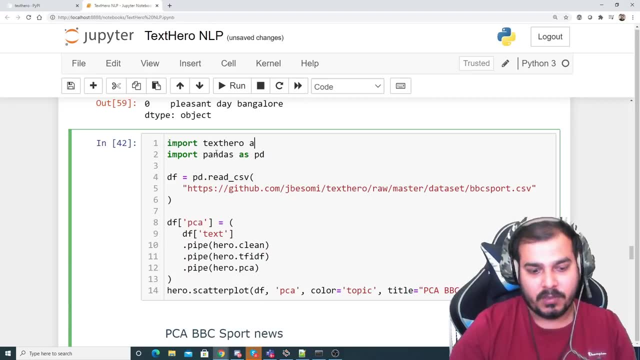 now one example where i'll be showing you the main power of this particular library: uh, as shown right. so if i write import text hero as hero right now here, what i'm doing? first of all, i'm reading this particular data set and i will be performing all the steps step-by-step. 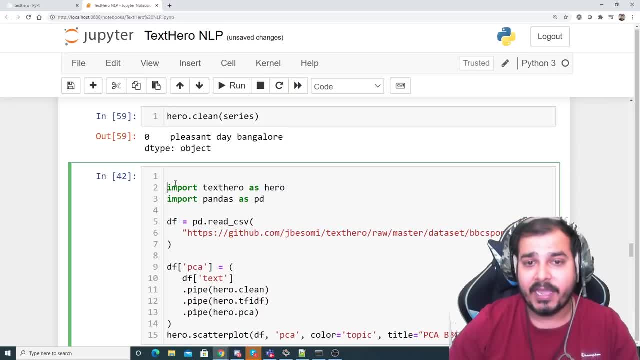 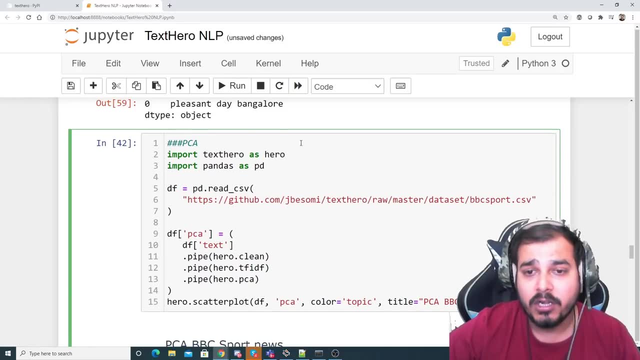 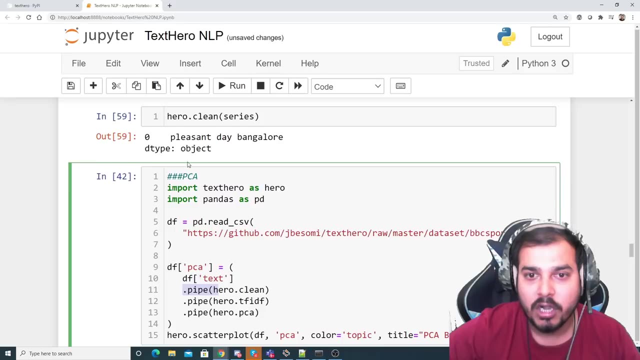 now see in this entire code, we are actually performing pca- principal component analysis. that basically means dimensionality reduction. now, in order to perform it, first of all i'm reading this data set, then i'm taking this data set and creating a pipeline where we are doing heroclean. heroclean is nothing, but we are cleaning. 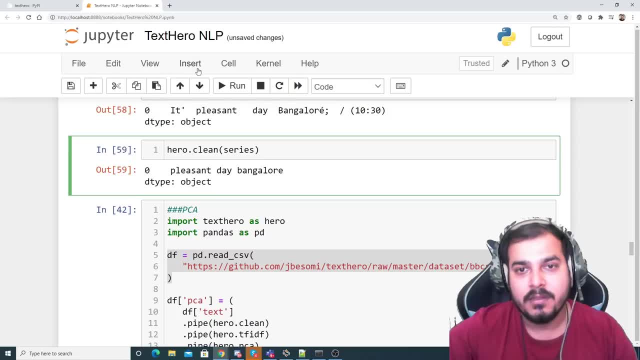 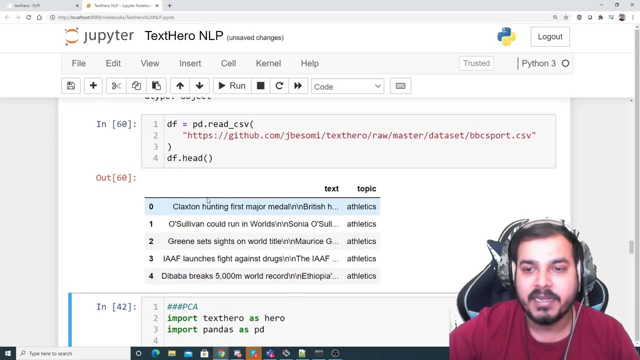 all the data. if you really want to check out what is this particular data, i will just show you. so here i'm going to execute it. let me write dfhead. so here is my entire data set. see, this is my text data and this is basically my topic, based on this. 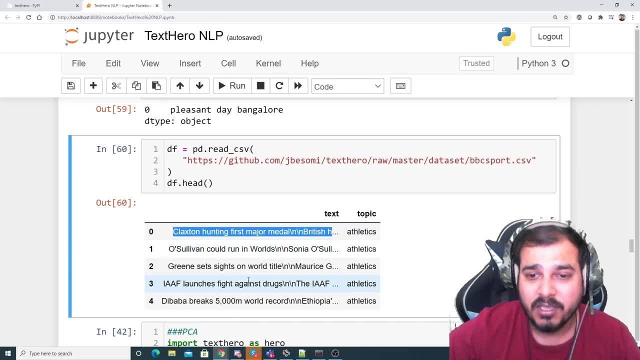 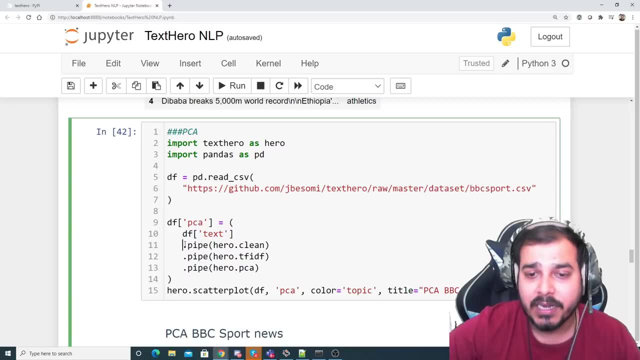 particular text data. we need to classify this particular topic, you know. so that is what probably this entire problem statement is all about. so what i'm doing over here, we are taking the text data, we are cleaning it and then we are doing tf, idf, where we are vectorizing it in this particular 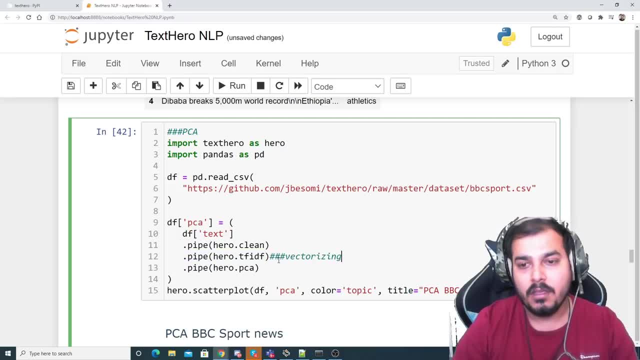 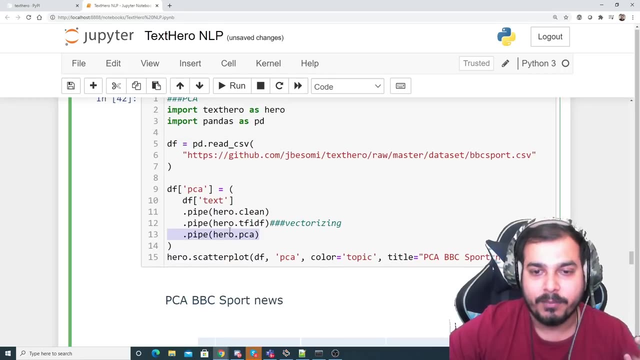 step we are vectorizing, right, converting those text into vectors, and then finally, we are using pca and we are basically converting that, probably, into two dimensions. this default converts into two dimension all the vectors. it will try to convert into two dimension. so here your entire text, pre-processing: 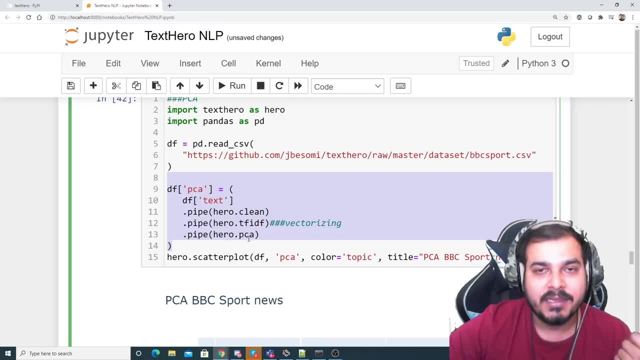 plus, your text is getting converted into vectors, and then dimension reduction is also getting applied. now, once after this, there is also a scatter plot inside this particular library, that is text hero. here you are just giving your df and you're saying that, based on the pca, okay, and then here, pca. 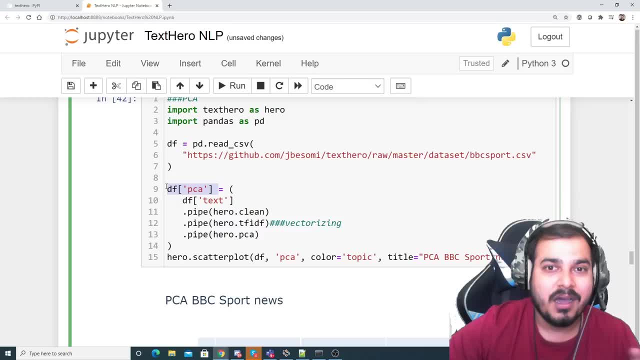 df of pca. see, guys, if i execute this, df of pca will be your another field, you know. uh, probably this will be your new column, right? so here i'm taking df, pca and color is equal to topic and this, once i execute it here, you will be able to see the entire. 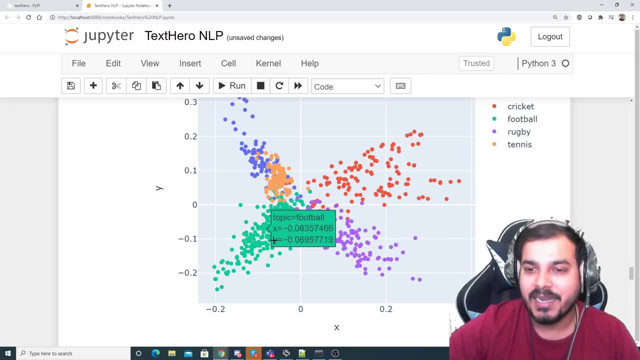 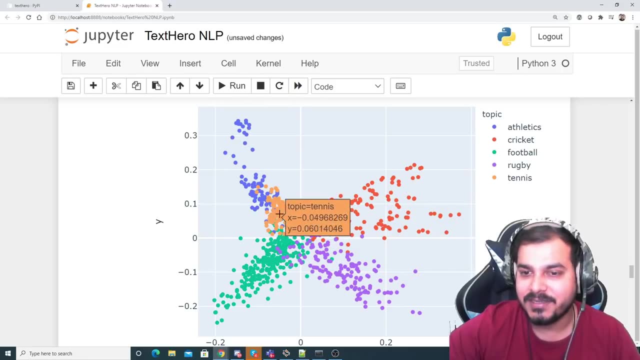 uh, text data in two dimension and how amazing little is being able to group it. you can see over here: cricket: it's this side. athletic is this side. football is this side. tennis is this side. there's a lot of overlapping of tennis and probably blue color is athletics. 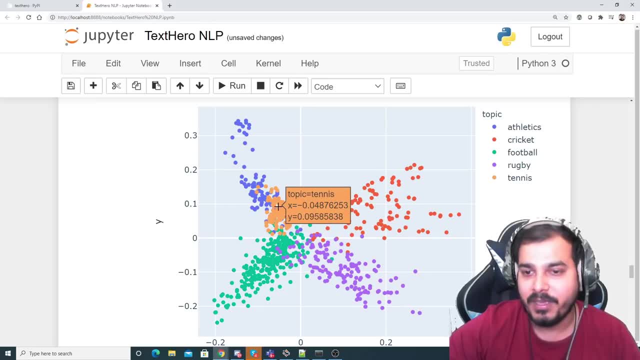 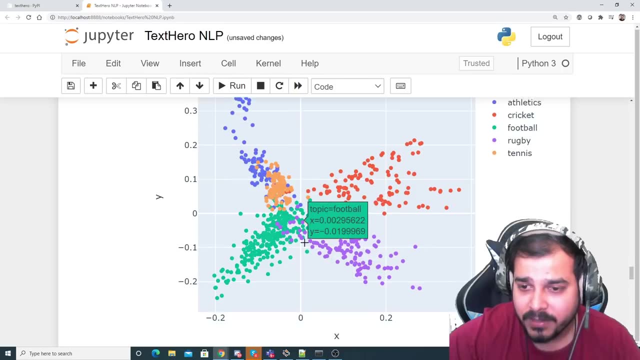 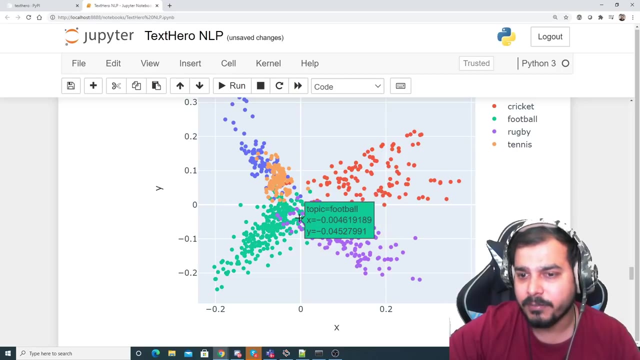 because probably, of people who are playing tennis, maybe, maybe, athletes. uh, so because of that, most of the text data are also resembling over here. yes, there are also some overlapping with respect to cricket and rugby. similarly with respect to this football and rugby. okay, because rugby is also. 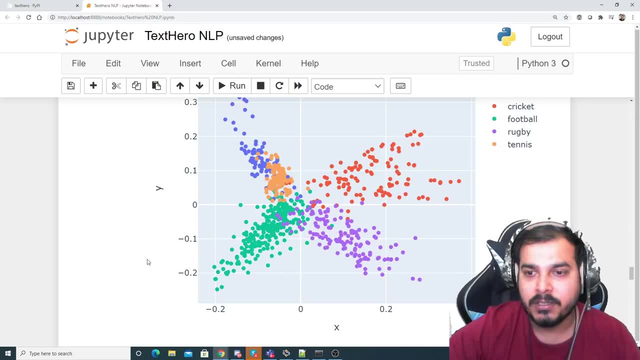 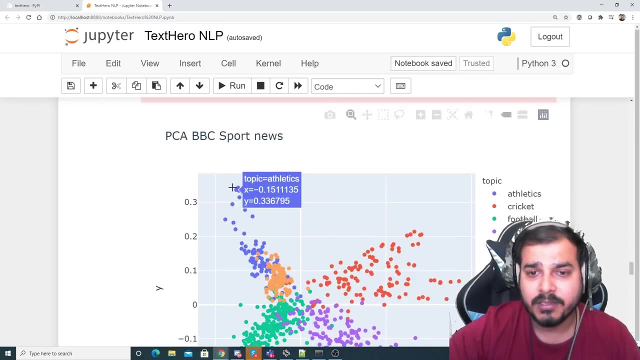 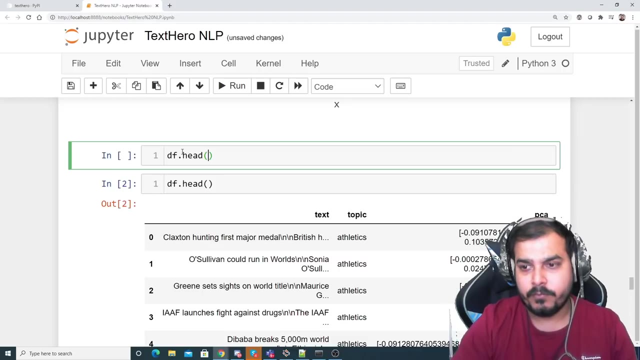 kind of football, american football. we basically say because in us and all we they say as american football. okay now one more example. uh, instead, here we have just done pca, right, we have just done pc, if you want to really see. uh, df dot head. so this is your pca, which is basically having two coordinates, two dimension. 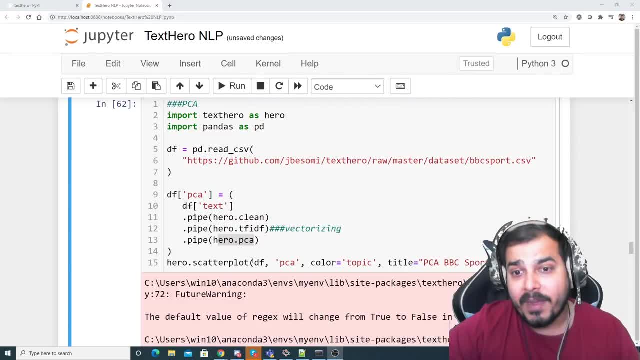 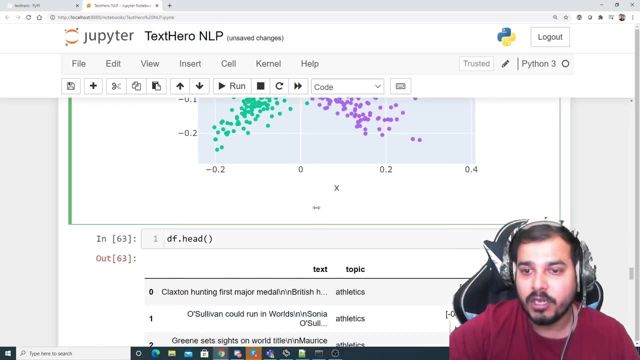 all this text vector has been converted into two dimensions. so, by default, when we are applying this pca, it is actually converting all the vectors into two dimensions. okay, so here it is all your data. similarly, let's take one more example again, guys, this entire notebook file will be given in the github link. 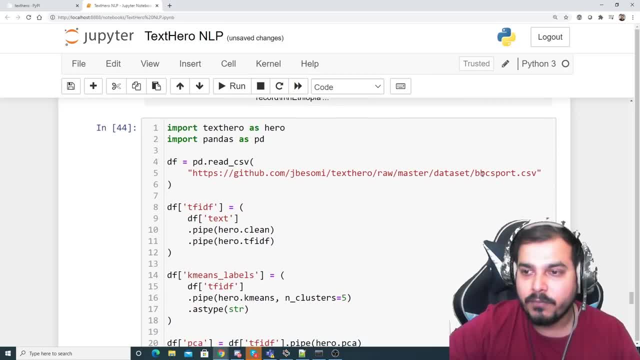 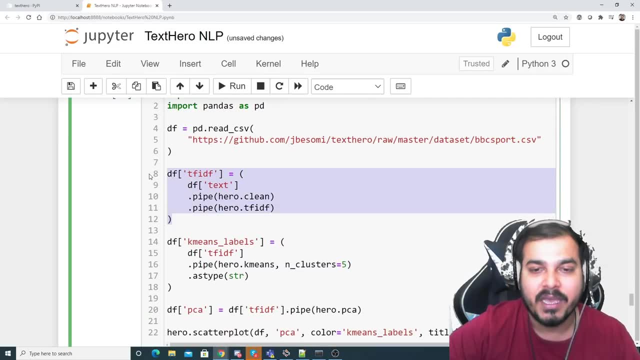 the link will be given in the description. so here what all things we are doing. we are reading this bbc sportcsv file. we are converting. first of all, we are doing this tf idf for tf idf. we are uh doing, we are con, we are using these two pipelines. one is clean. 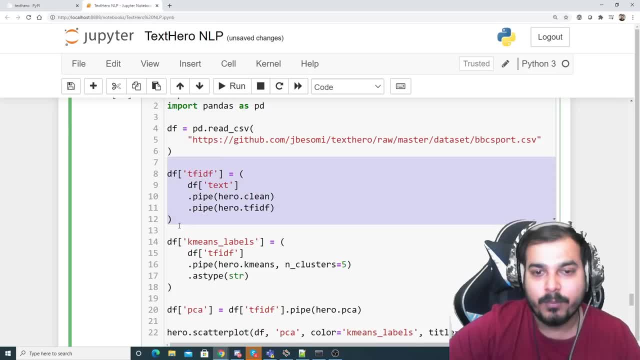 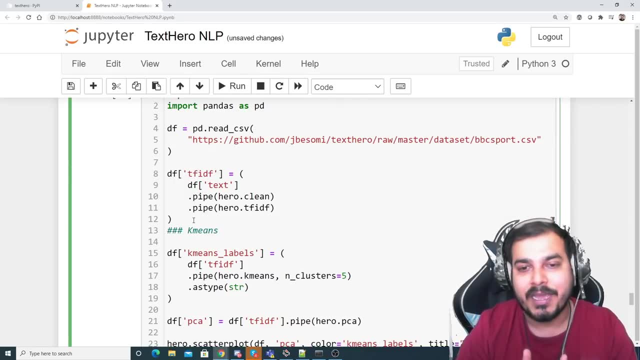 and one is herotf idea. after this we are applying k means, so that basically means we are trying to group it. we are not now trying to reduce the dimension, but instead we are trying to reduce the dimension, but instead we are trying to reduce the dimension, but instead we are.